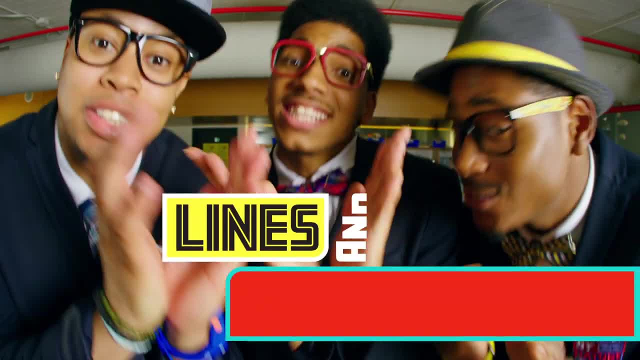 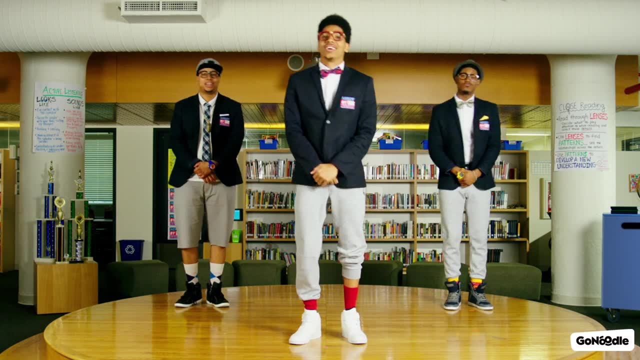 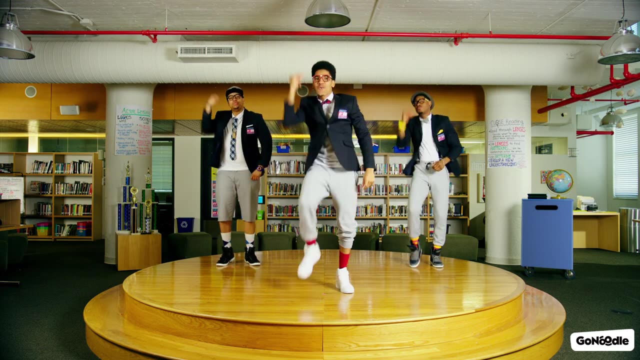 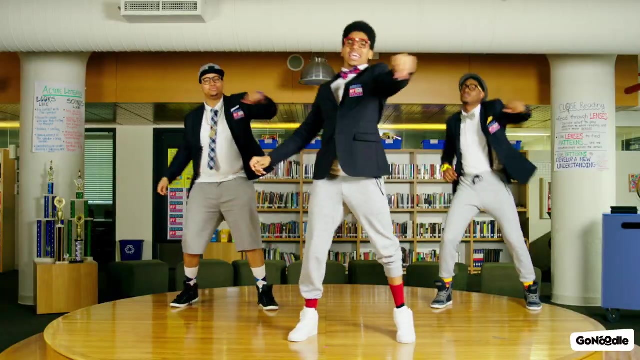 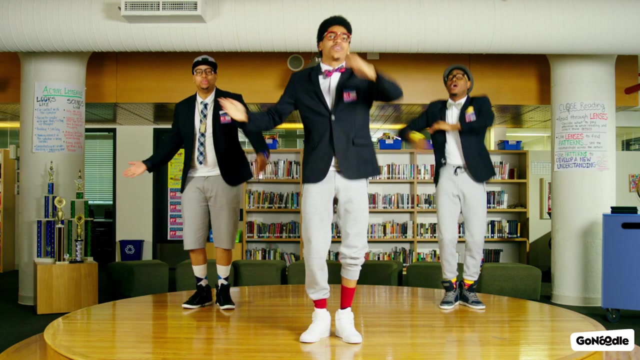 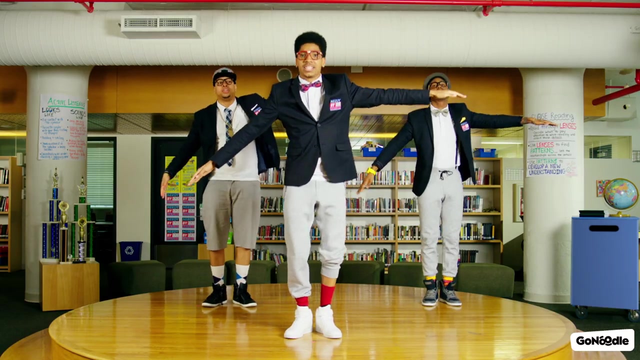 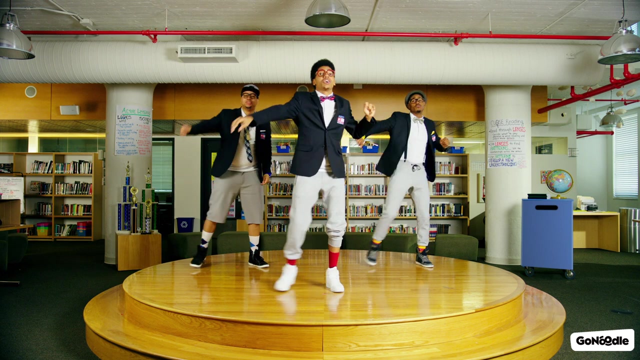 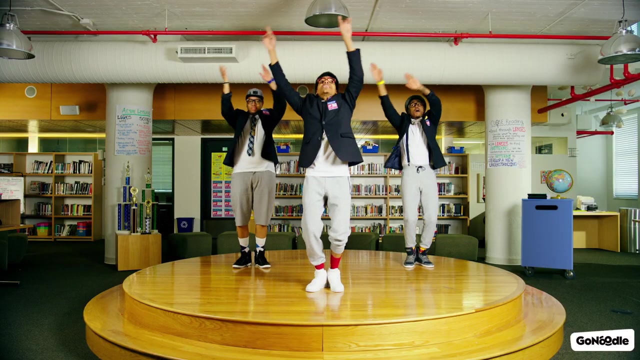 Lines and angles, angles and lines. get your groove on, and I'ma get mine. Lines and angles, angles and lines. let me see that angle looking mighty fine. Check it out, my peeps. lines and angles are a breeze, cause you know that right angles are 90 degrees. If it's less than 90, then that angle is acute. Kinda like a right angle. God, step on by a boot. Here's another angle that I've got to introduce. If an angle's more than 90, then we call that thing obtuse. A straight angle. it's looking super flat. It's 180 degrees. Come on and stretch it out like that. A reflex angle greater than 180. Here's the plan. whip your arms around like this so you can do the Pac-Man: 160 degrees is a full rotation Round the world and back to your original location. 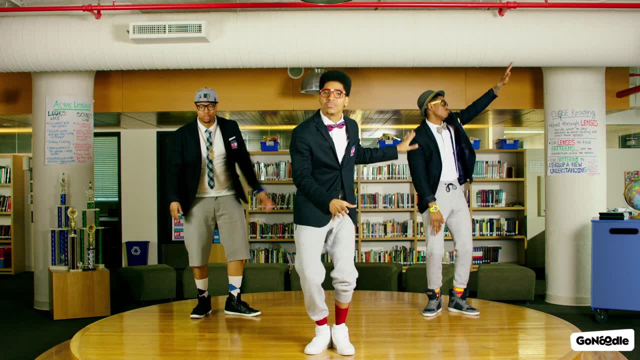 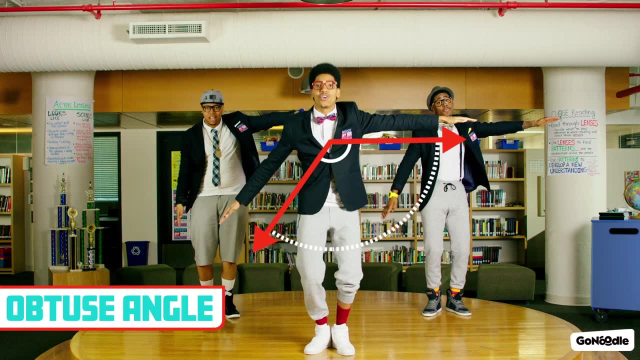 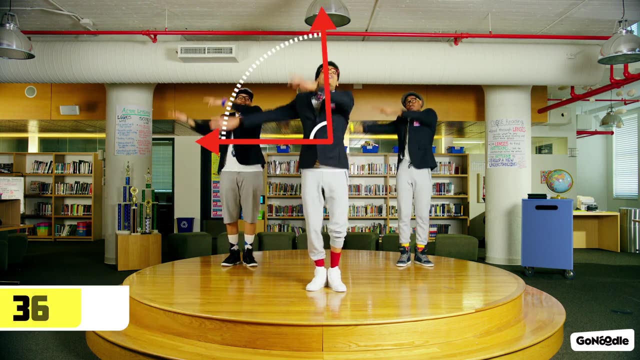 Alright, let's do these angles. Here. it is Right angle, right angle, acute angle, acute angle, obtuse angle, obtuse angle, straight angle, straight angle, reflex angle, reflex angle, full rotation, full rotation. nerdy by nature. 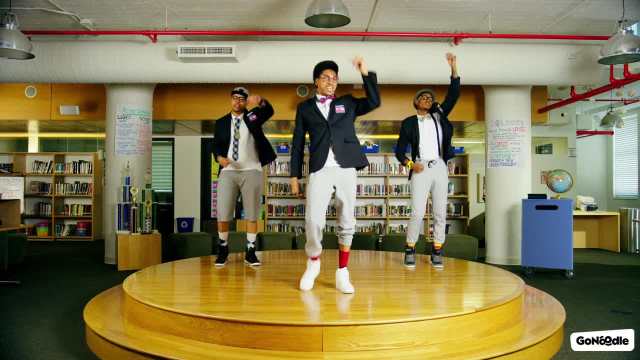 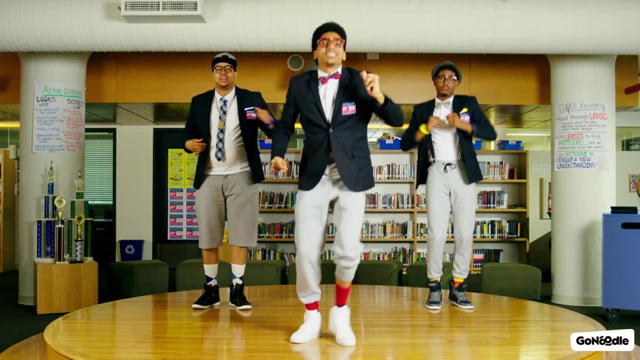 Lines and angles, angles and lines. get your groove on and I'ma get mine. Lines and angles, angles and lines. let me see that angle looking mighty fine. Two lines on the same plane. what you call them, Can you tell? they never intersect. yo, That means they're parallel. 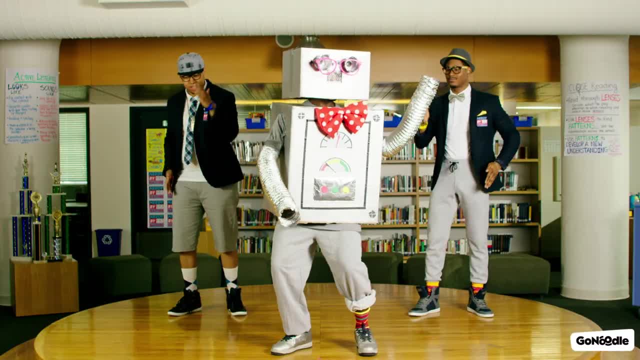 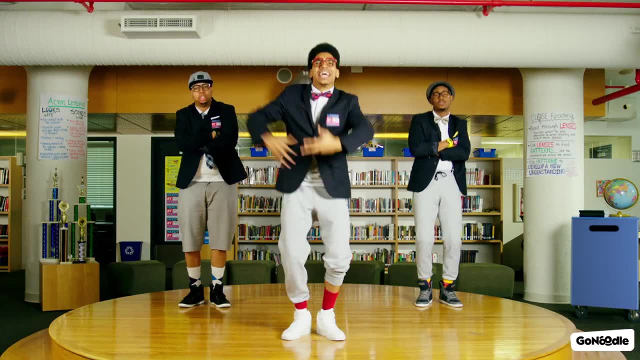 When lines meet at right angles, it's so particular, Like when I do the robot, yo I'm on perpendicular intersecting lines, It's what you call it. when they cross, when I cross my arms like this, I feel like I'm a boss, He's a boss. 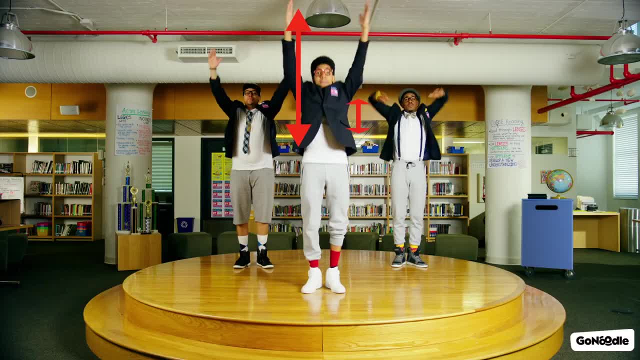 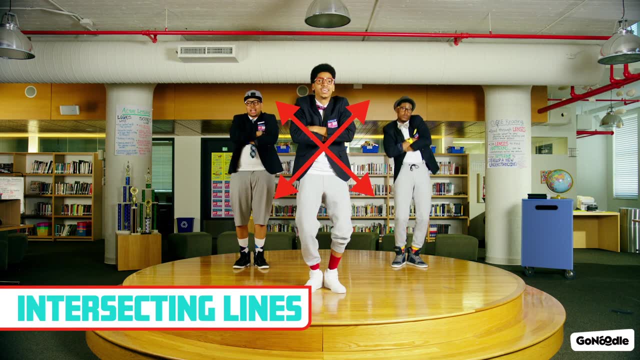 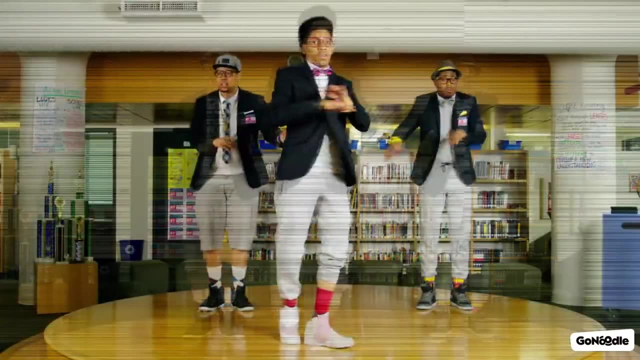 Alright, let's hit these lines. Here we go. Parallel lines, parallel lines, perpendicular lines, perpendicular lines, intersecting lines, intersecting lines. Rewind that one more time. My eyes don't know when. now Let's go. 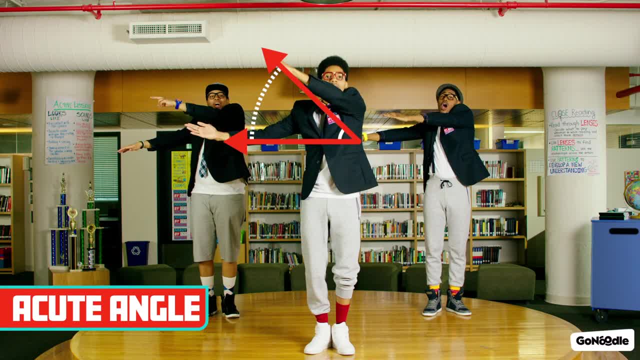 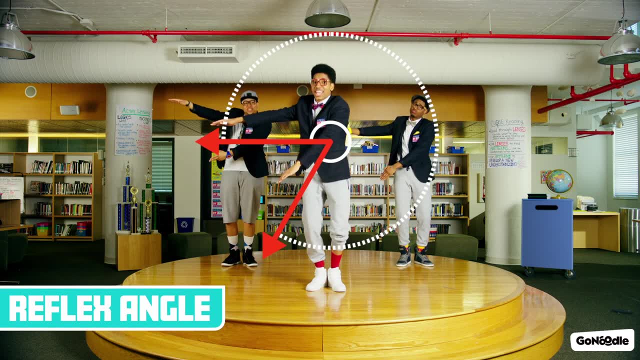 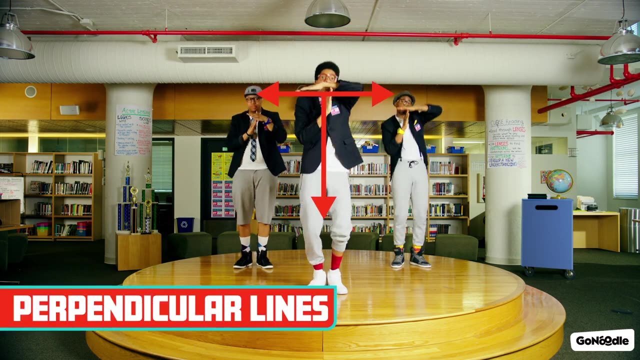 Right angle: right angle- acute angle. acute angle- obtuse angle. obtuse angle. straight angle. straight angle reflex angle. reflex angle. full rotation. full rotation- Parallel lines, parallel lines, perpendicular lines, perpendicular lines, intersecting lines, intersecting lines.